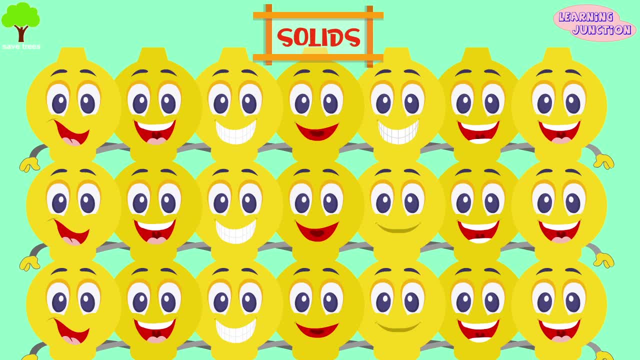 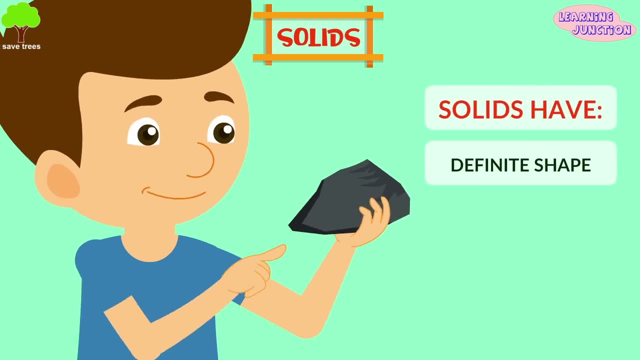 but they are fixed in their place. Due to this, particles in a solid have a little vibration, but they are fixed in their place. Solids have very small amounts of kinetic energy. Solids have a definite shape, as well as volume and mass. 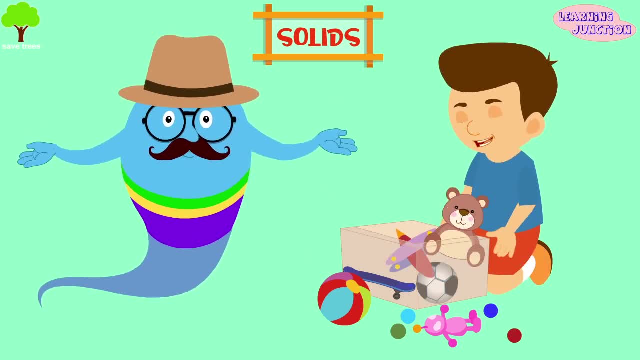 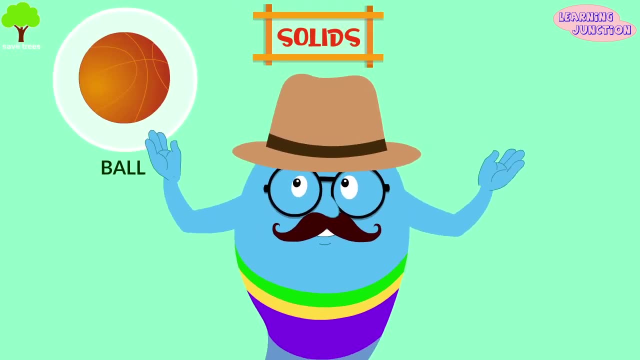 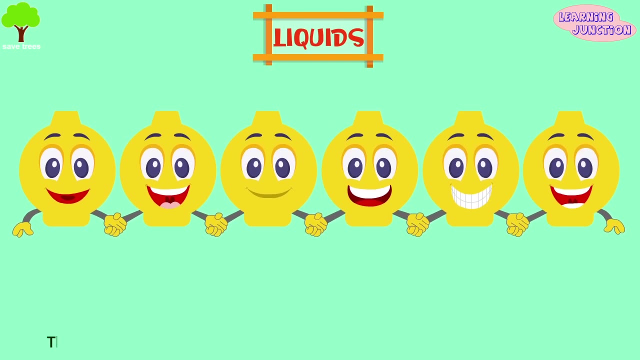 Solids do not comply to the shape of the container in which they're placed. Some examples of solids are the ball you were playing with a chair, books and dice Liquids: In a liquid state, the particles are more loosely packed. 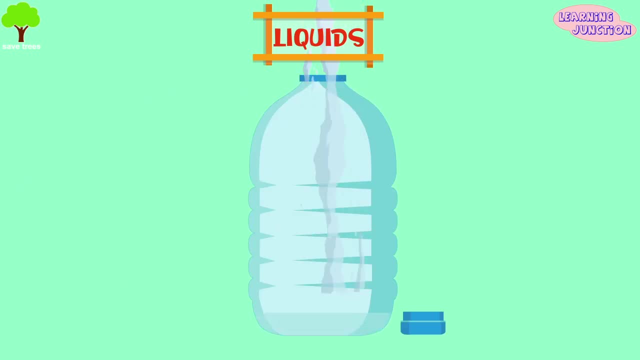 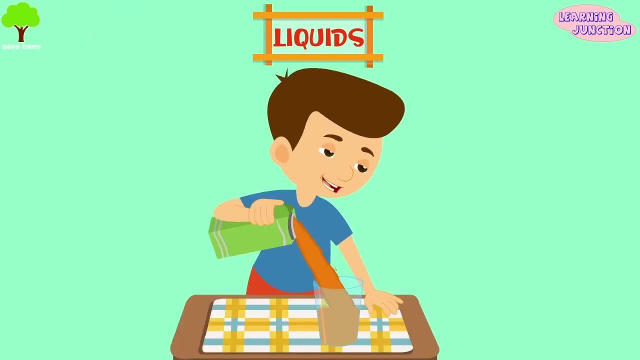 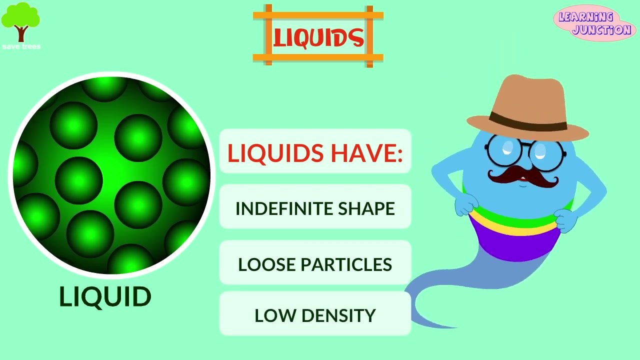 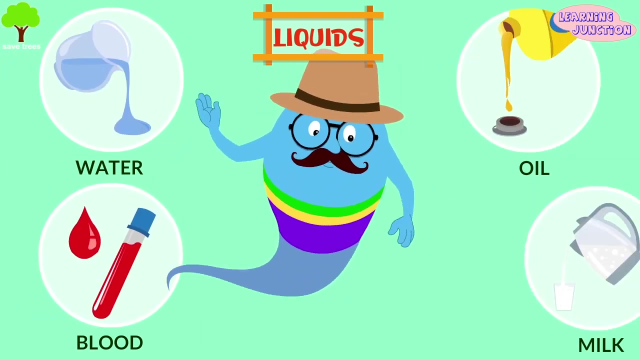 And they're able to flow around each other. It gives the liquid an indefinite shape. Therefore, the liquid will comply to the shape of its container. Because the particles are loosely packed, liquids have low density. Some examples include water, blood oil and milk. 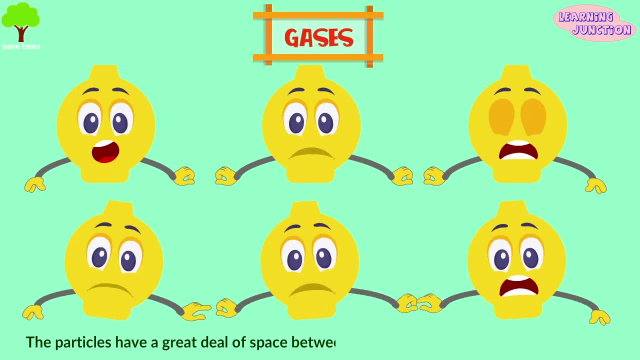 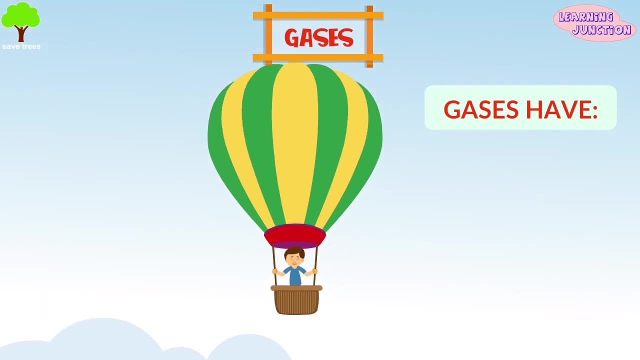 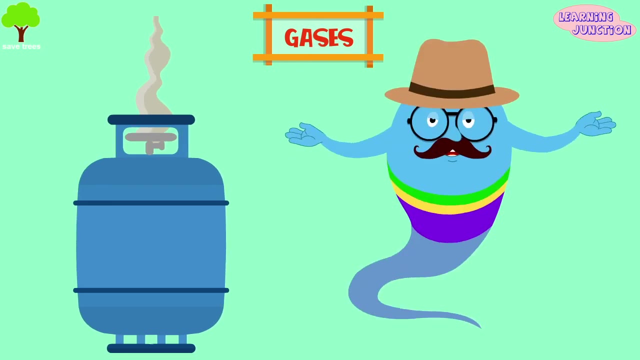 Gases. In this state, the particles have low density, They have a great deal of space between them and have very high kinetic energy. A gas has no definite volume or shape. Gases can fill up the entire volume or space of a container, irrespective of the size of the container. 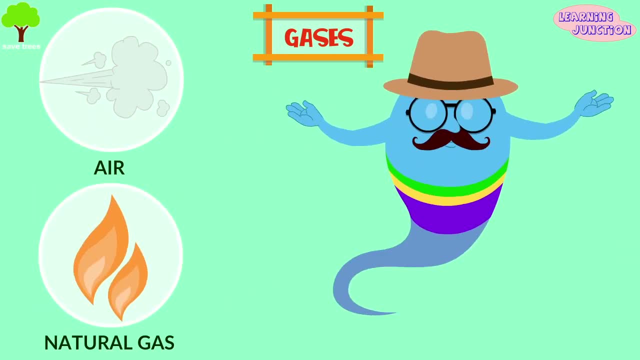 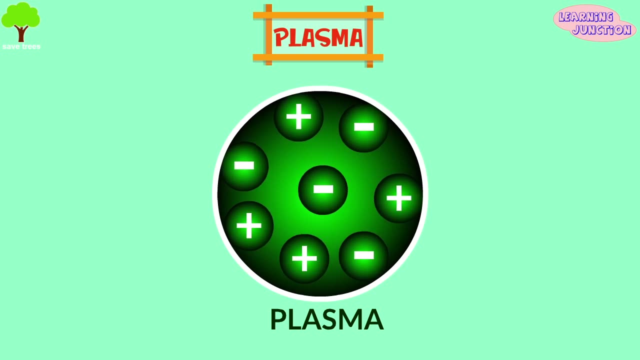 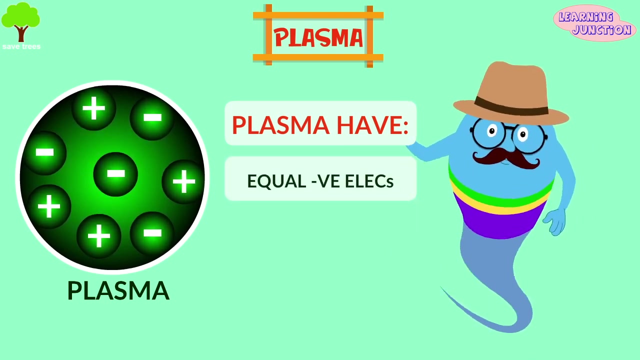 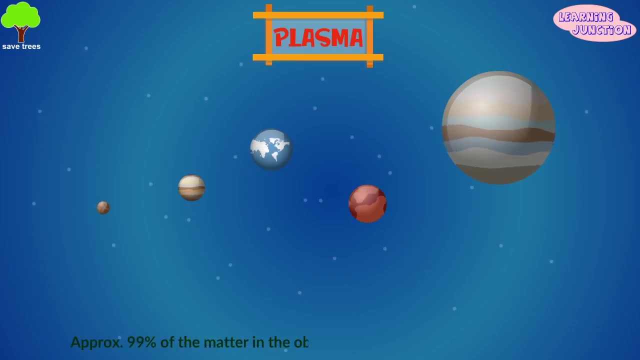 Some examples include air, natural gas, hydrogen and water vapor Plasma, Plasma A. plasma is a warm ionized gas consisting of almost equivalent numbers of negatively charged electrons and positively charged ions. It is estimated that approximately 99% of the matter in the observable universe is in the plasma. 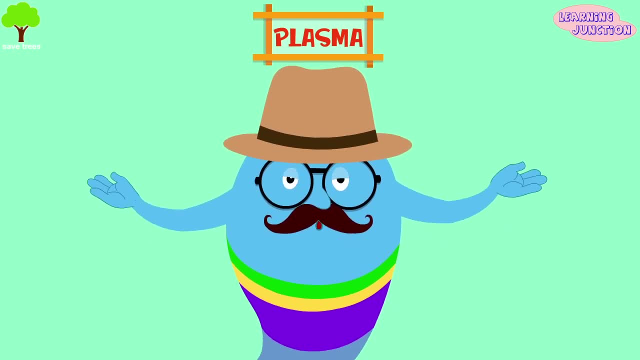 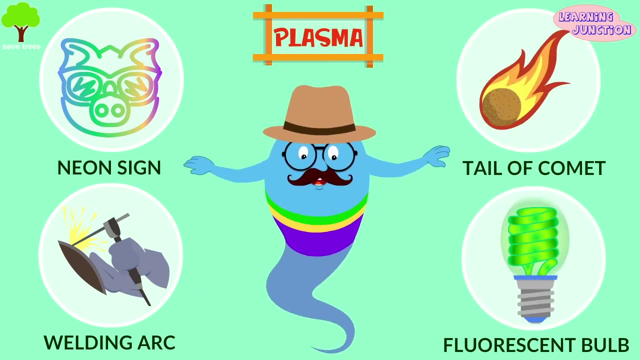 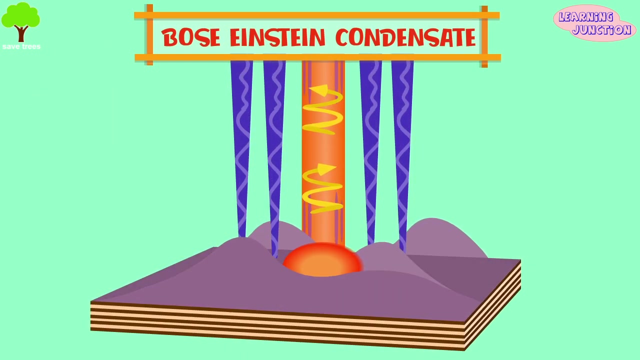 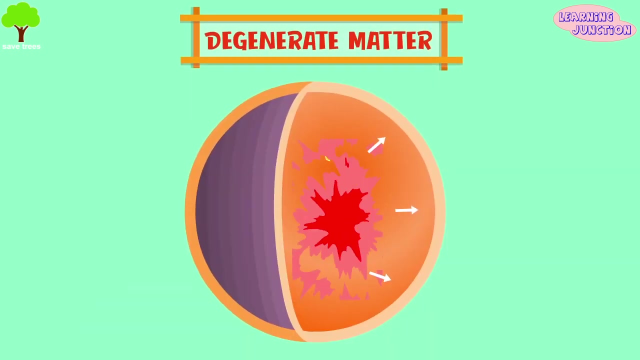 state. Some examples include neon signs, welding arcs, the tail of a comet and fluorescent lights. Some other states of matter are Bose-Einstein condensate. It is a state of matter that occurs very, very close to absolute zero. Degenerate matter. 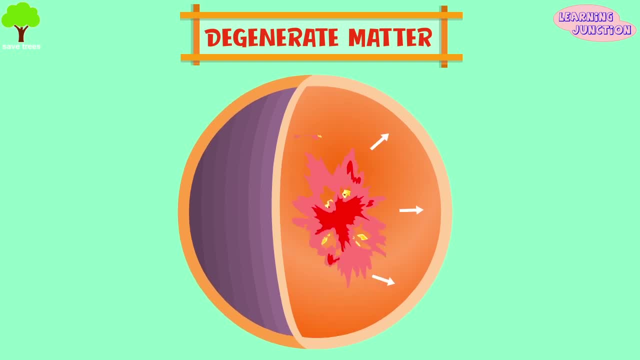 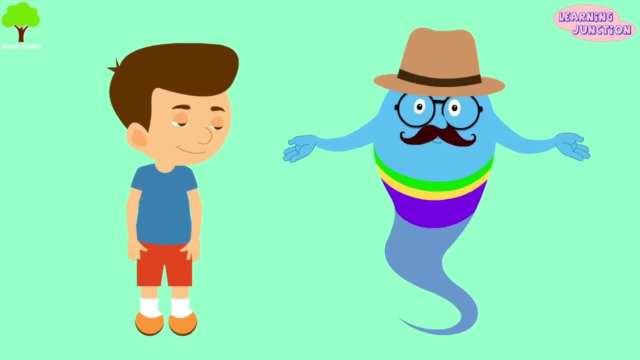 It is the supremely compressed state of matter which often exists in the cores of massive stars. Now you know a lot about the states of matter. Stay tuned for more videos. Bye-bye.